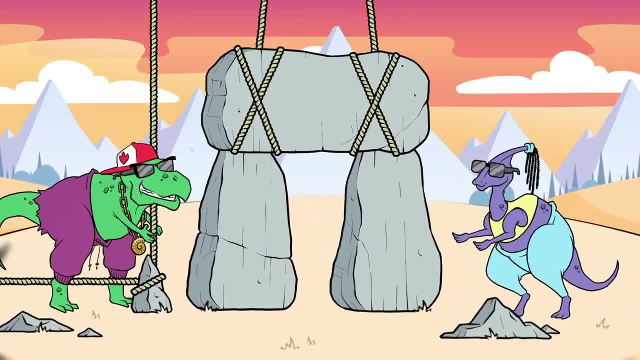 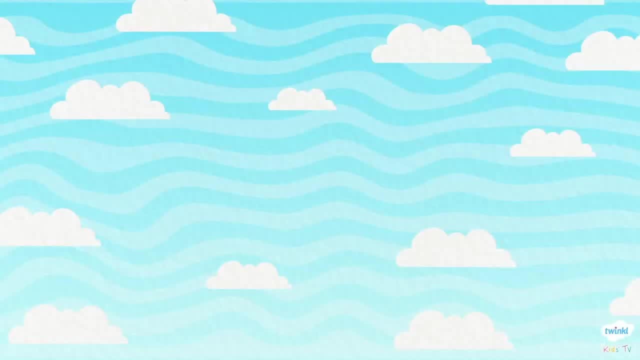 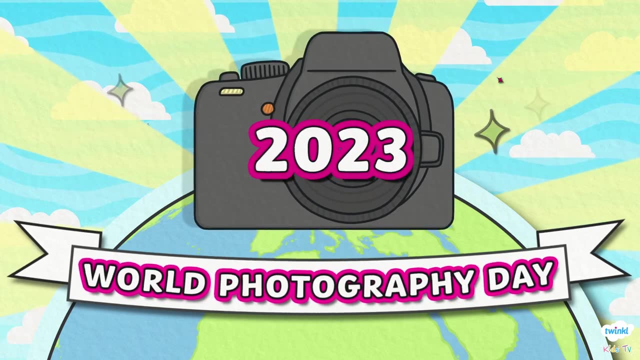 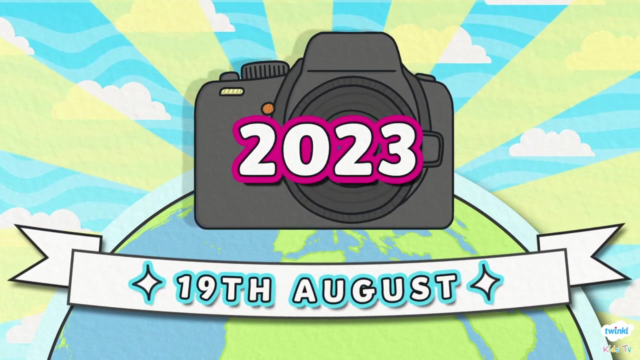 World Photography Day is an annual celebration of the art of photography. In 2023,, World Photography will be celebrated on the 19th of August. Each year, there is a new theme to the day. In 2023, the theme is Understanding Clouds. 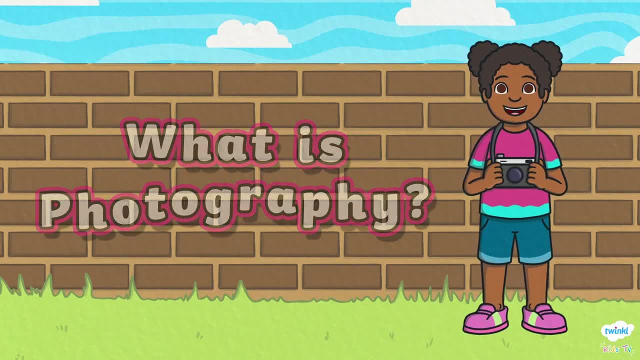 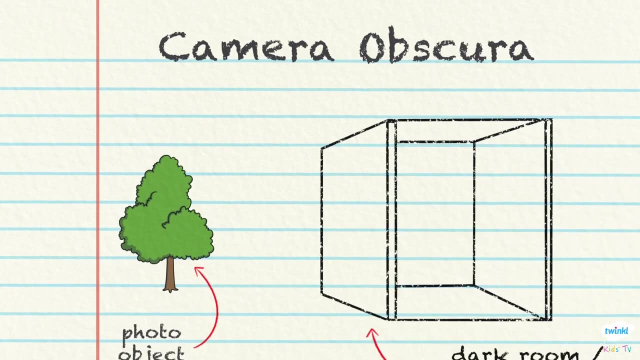 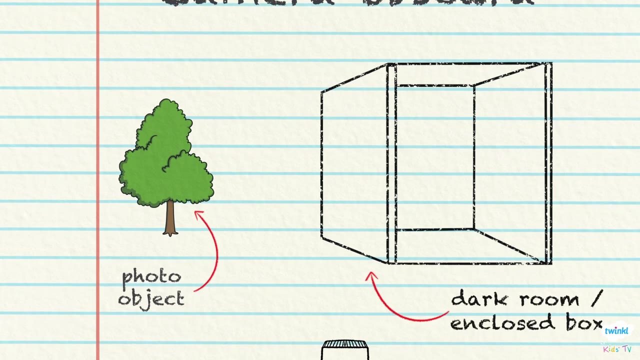 What is photography? Photography is the art of capturing images using a camera. The first camera-like device to be invented was the camera obscura. This was a device made up of darkened rooms or enclosed boxes with a small opening on one side. When light passed through, it projected a blurry image onto the screen. 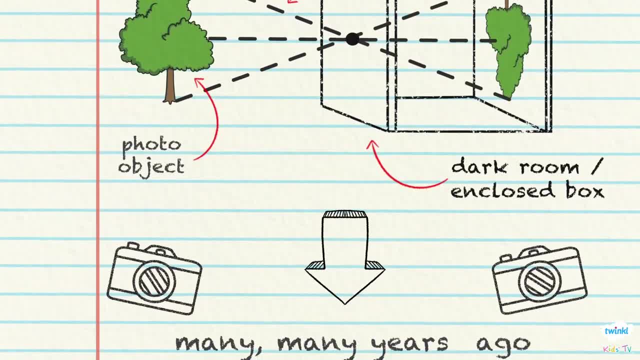 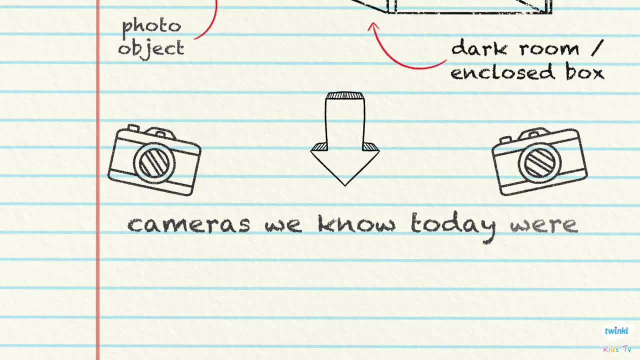 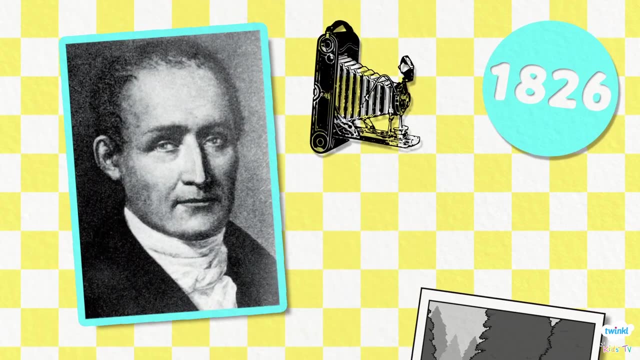 The camera obscura was invented many, many years ago, dating back to the 5th century, But the cameras we know today were first invented much more recently, in the 19th century. In 1826, Joseph Nicephore Niepce was the first person to permanently capture an image. 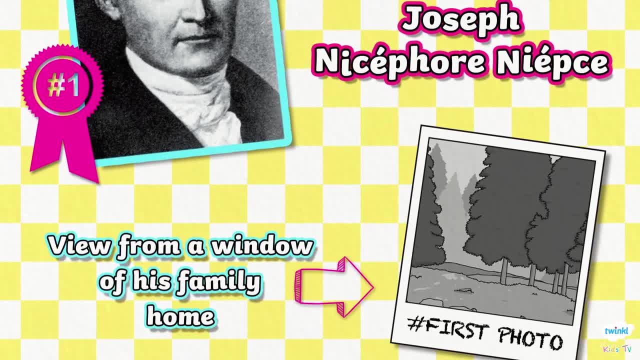 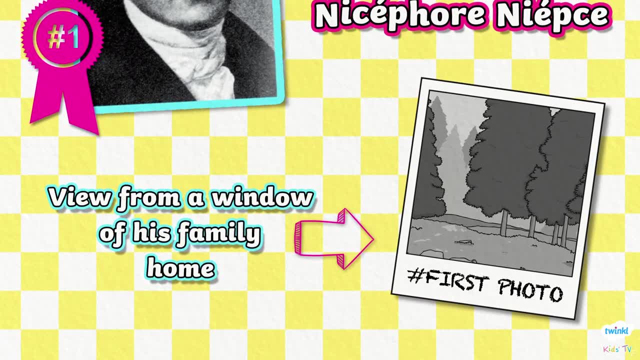 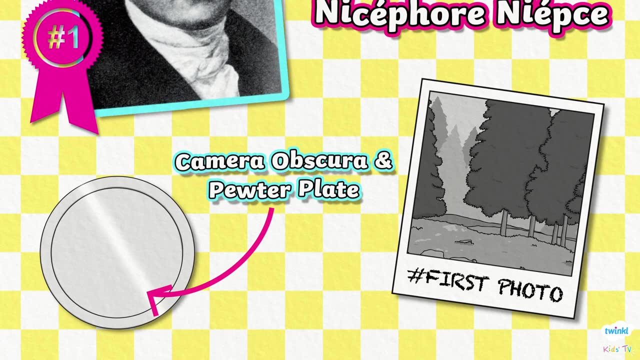 Taken with a camera. The first photograph ever taken was by Joseph Nicephore Niepce and was an image of the view from a window of his family's home. He used the camera obscura and a pewter plate. The plate was covered in a light-sensitive material that fixed the image to the plate. 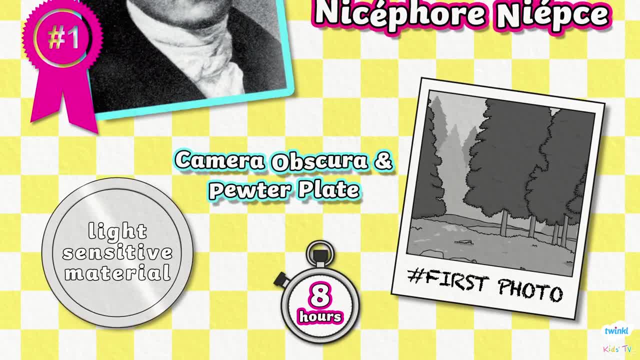 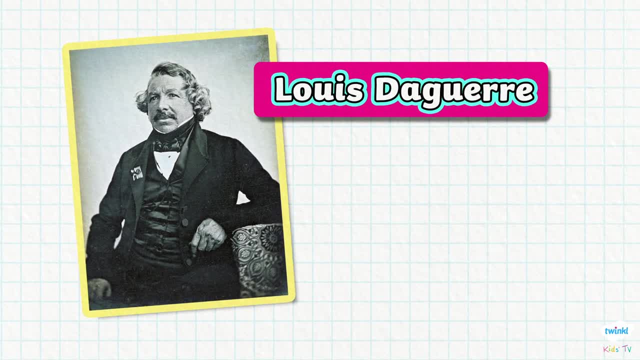 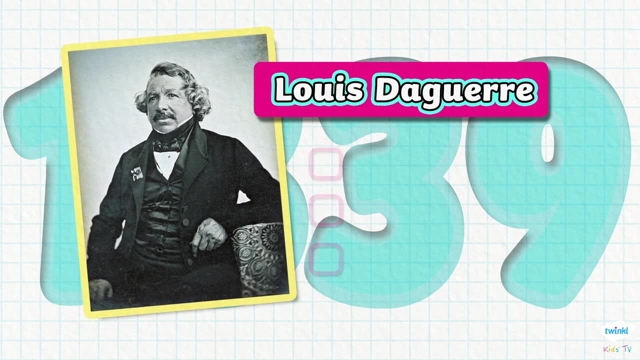 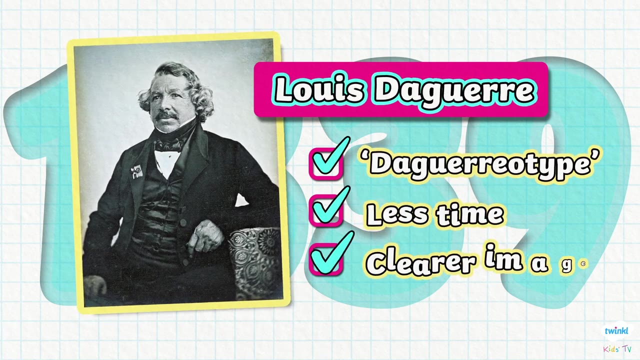 This process was very clever but took over eight hours and the image was not very clear. Niepce's associate, Louis Daguerre, was inspired by his findings In 1839,. Daguerre went on to develop the Daguerreotype process, which took much less time than the original process and made clearer images. 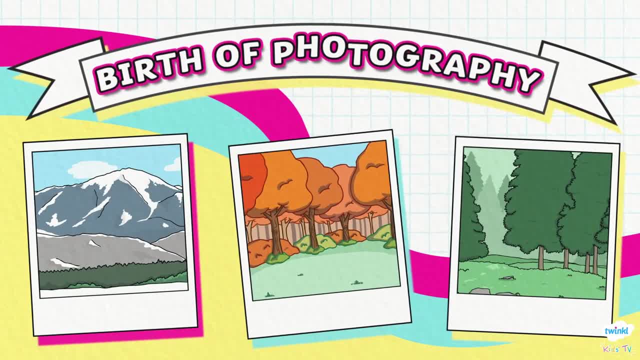 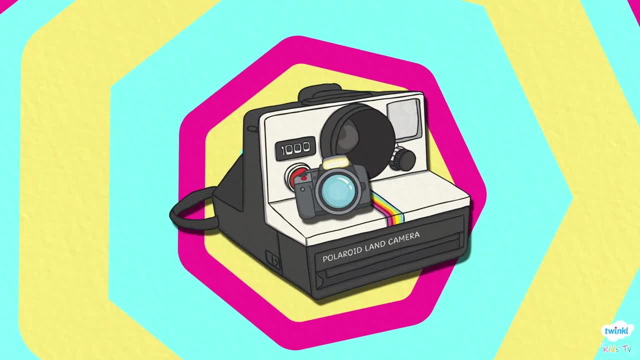 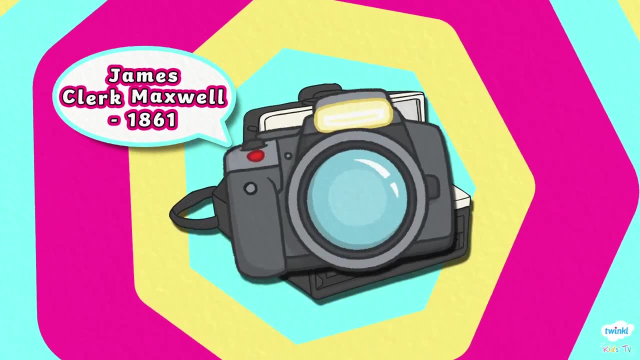 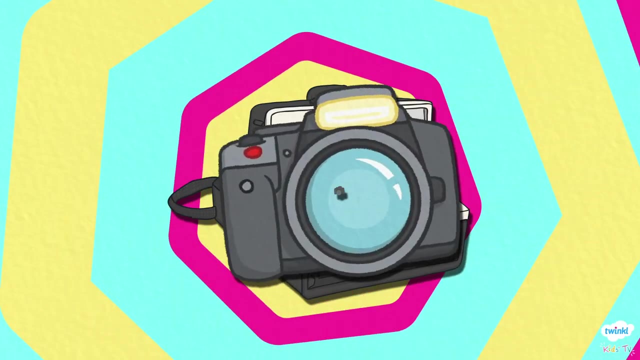 This was considered the birth of photography and is the reason we celebrate World Photography Day on the 19th of August. The camera was developed several times over the years, including colour photography by James Clerk Maxwell in 1861, and new processes including photosensitive paper, wet plates and more, to make the exposure time less and the images clearer.